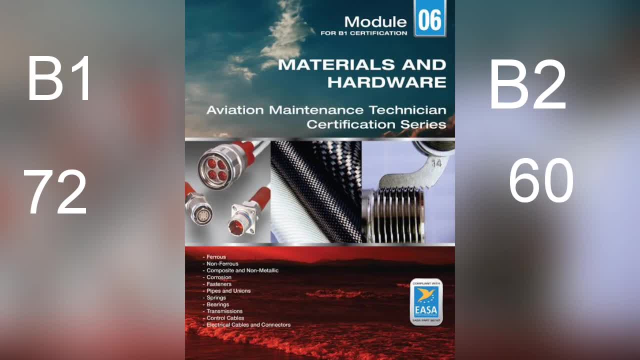 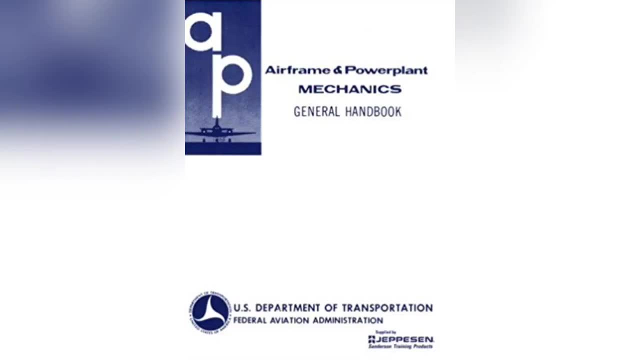 Equally important for B1 as well as B2.. 72 marks for B1 and 60 marks for B2.. This module is clearly important for both the streams, 9a being the core book for Module 6, and chapter 5, 6 and 7 being the only chapters that you. 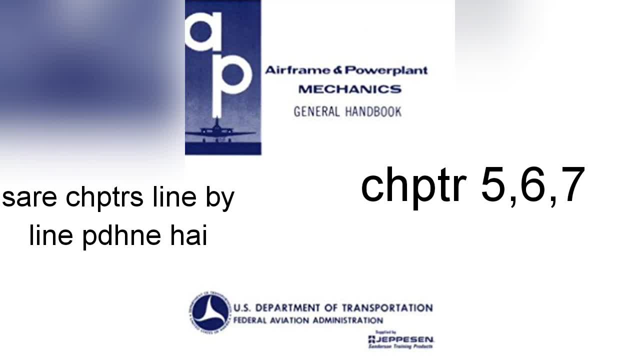 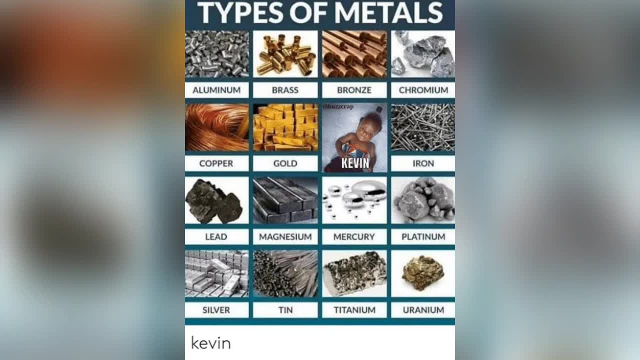 need to study from this book line by line, because this book is the most important book of all. Now the second most important book after 9a is Aircraft: Materials and Processes by George F Tritterton. From here you have to study about specific materials and their processes. 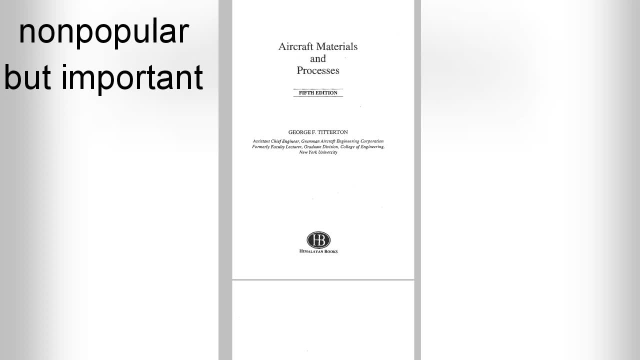 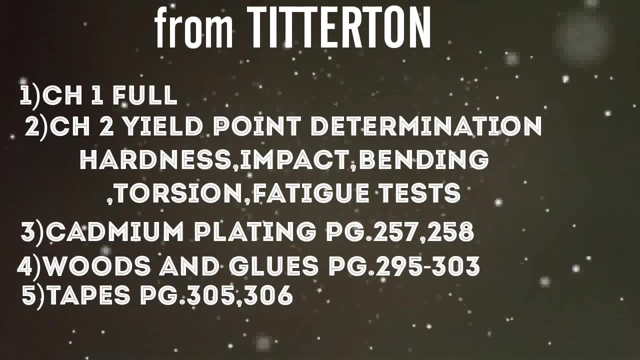 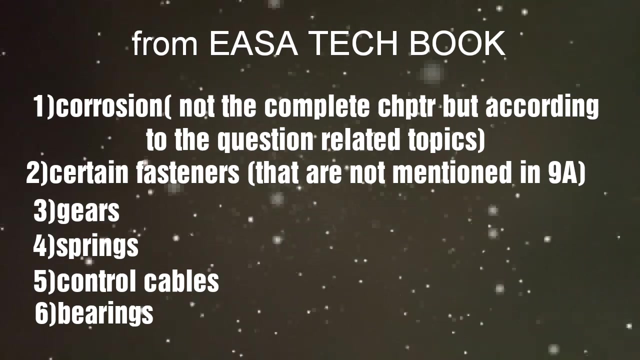 So here is another non-popular but important book for Module 6, and in the next clip I am going to tell you what specific things you have to cover. Let's get started. What am I supposed to do? I'm lonely here without you. 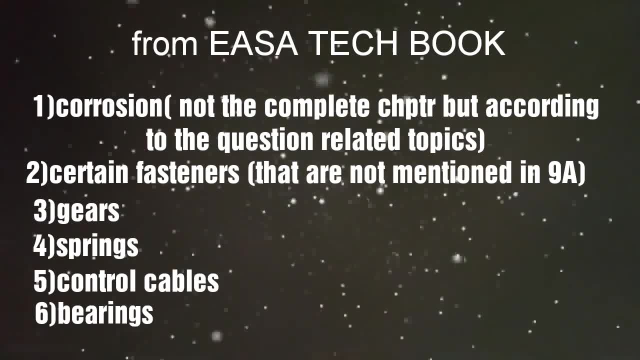 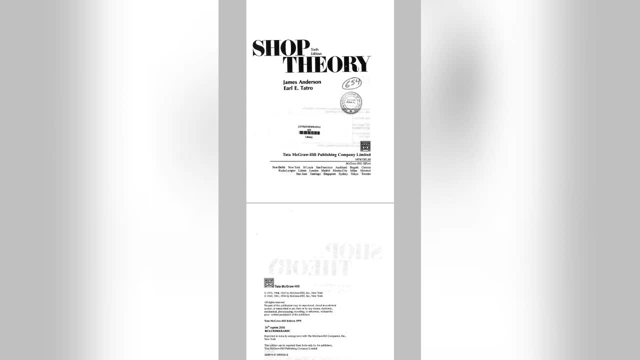 All these days are passing by Standing here. while you're living your life. I'm standing here. while you're living your life, I'm broken. So gears is the only topic that you have to cover from shop theory, because what's given in this book is completely different from what 9a and IASA book says. 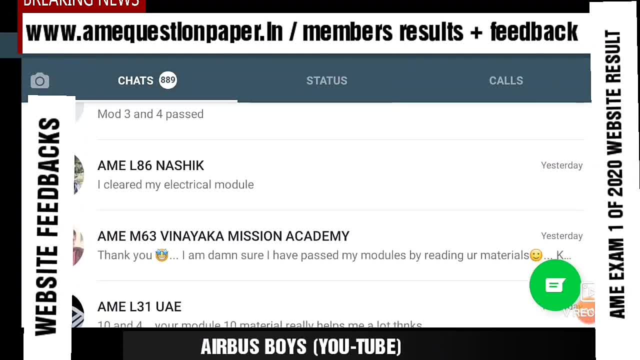 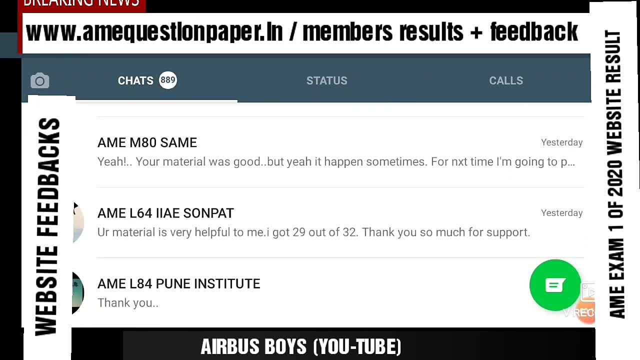 So, guys, this time, along with our video, we have also brought a bonus point. As you can see, on the top of your screen, there's a link of the site wwwamaquestionpaperin. By downloading and studying question paper from this site, about 900 plus students have reviewed of their 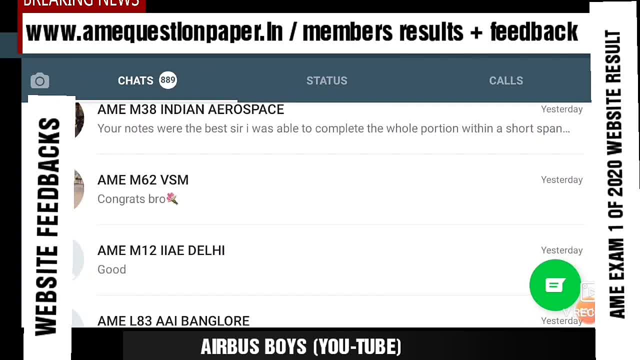 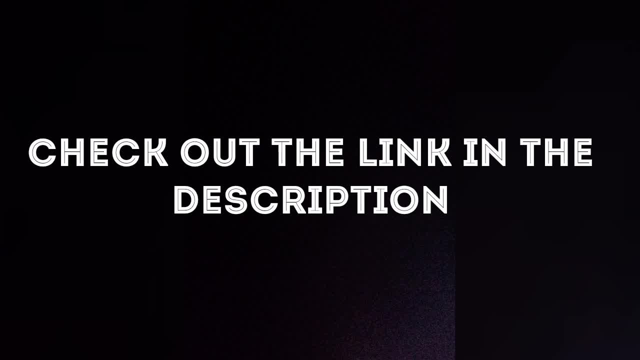 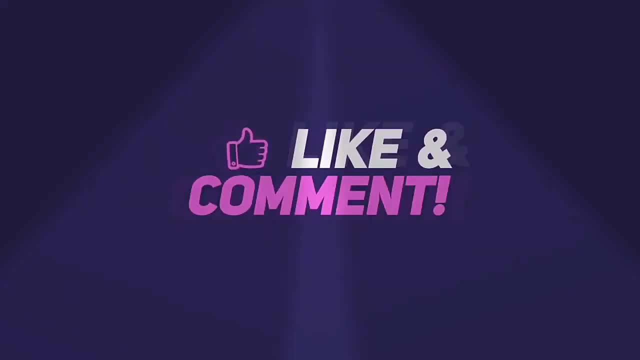 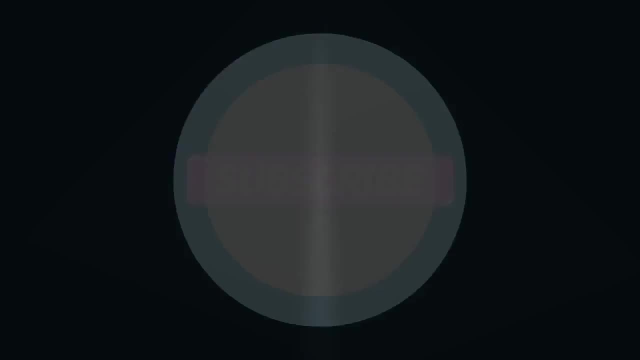 past. This was after speaking truthfully about social distancing and Champa Hey, last attempt. As you can already see a whatsapp chat containing 889 students who claim to be passed. Check out the link in the description box below. Okay, and Plz subscribe to this channel and Thankyou for watching this video. See you in the next one. Bye, bye.